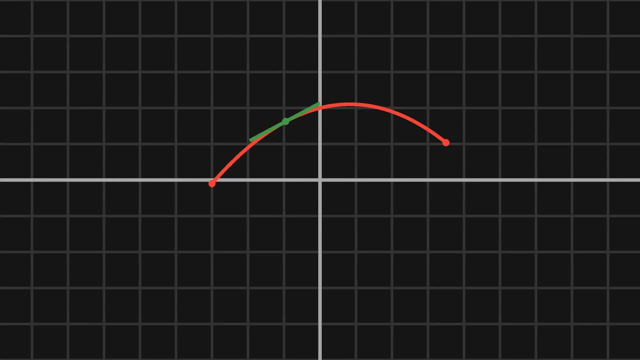 f just becomes a function in terms of x, and when we integrate over it, we're essentially summing all of its values over the curve y of x. While this may seem a little pointless now, it ends up being a very important idea. An example you may be familiar. 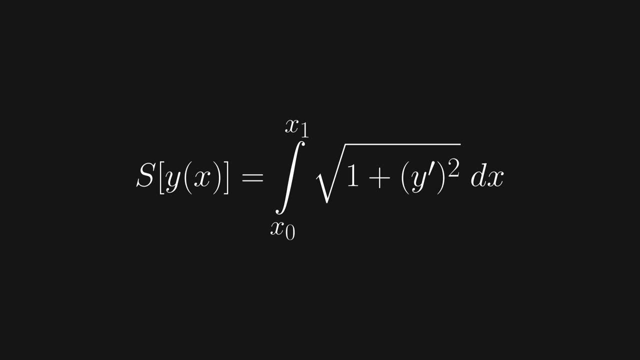 with is finding the arc length of a curve. We can write the arc length as the integral of the square root of 1 plus y, prime squared. Notice that this perfectly fits the form of j of y. Another problem you may be familiar with is the brachistochrone problem. You can write the time it takes to roll. 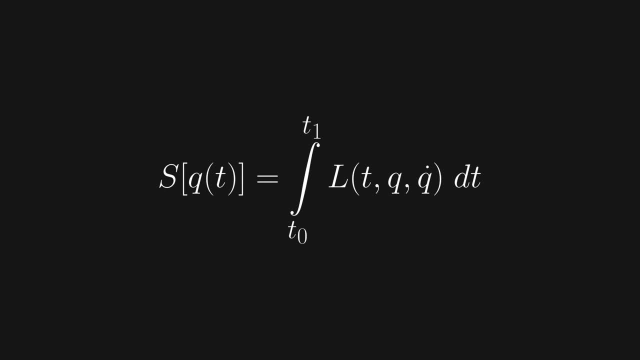 down a function as this integral. Another important example is found in Lagrangian mechanics. Lagrange managed to show that a particle will take a path where the integral of its kinetic energy minus its potential energy, commonly called the Lagrangian, is the lowest. This 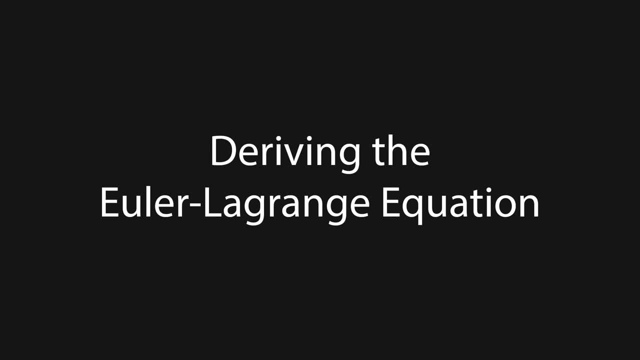 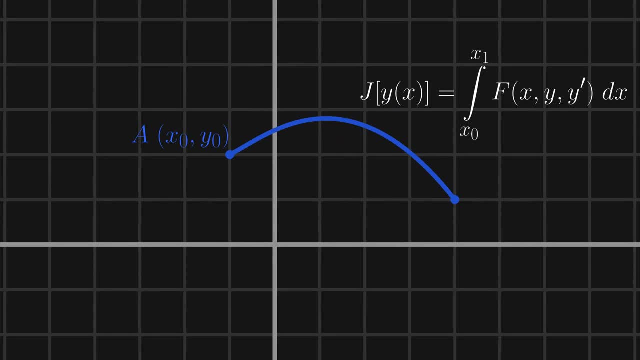 also fits the form of j of y. Now that you've gotten a sense for functionals, let's take a look at the central problem of the calculus of variations. For two points, a and b, there are an infinite number of curves that pass through them. 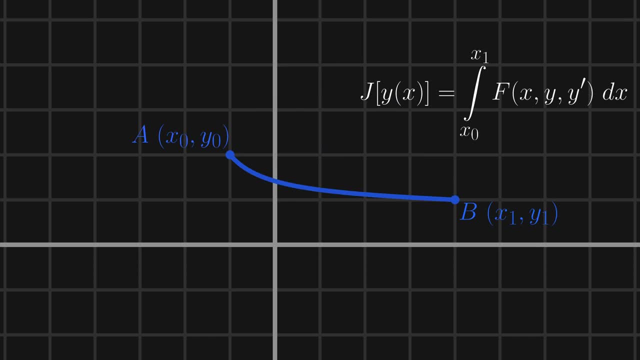 What we want to do is find the curve that is, the stationary point of j of y. Fundamentally, we're finding a curve between a and b that minimizes the integral of f over it. We're going to solve this in a similar way to how we solve the one-dimensional problem. 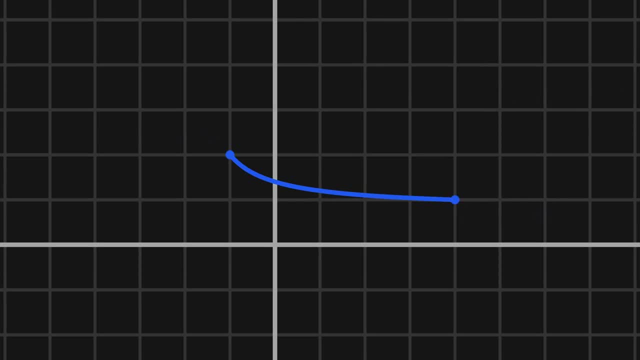 We're going to consider what happens when we add a small change to our input. but in this case any small change to our input would be a function. Let's say that y is an extremal of j of y. We let y-bar equal y plus epsilon times eta of x. Here, epsilon times eta is the small change in the. 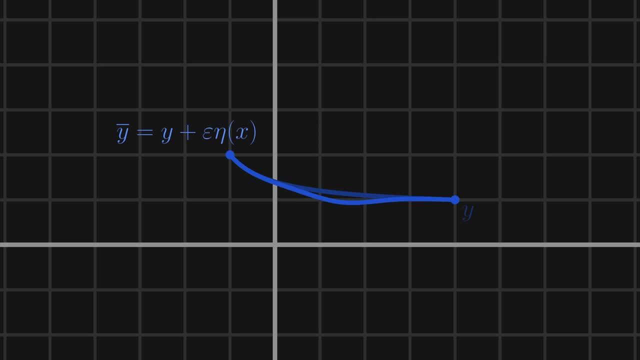 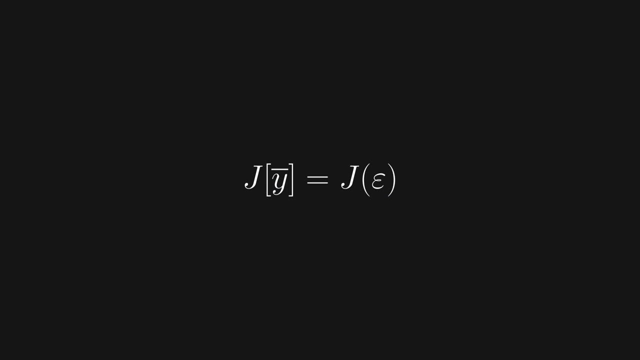 function. To ensure that y-bar still fits our boundary conditions, we need to let eta of x0 equal eta of x1 equals zero. Notice that j of y-bar is now just a function of epsilon, j of epsilon. Since epsilon equals zero is an extremal of j, we know that j-prime of epsilon at epsilon equals zero. 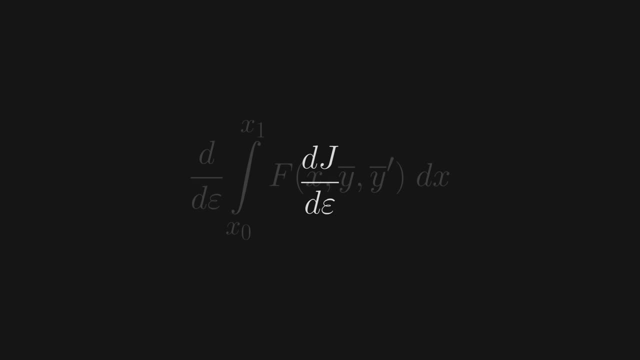 equals zero. Let's pay attention to simplifying dj d epsilon From Leibniz' rule. we can rewrite this as the integral of partial f partial epsilon from x0 to x1 dx. Using the multivariable chain rule, partial f partial epsilon becomes partial f partial y-bar times. partial y-bar partial epsilon. 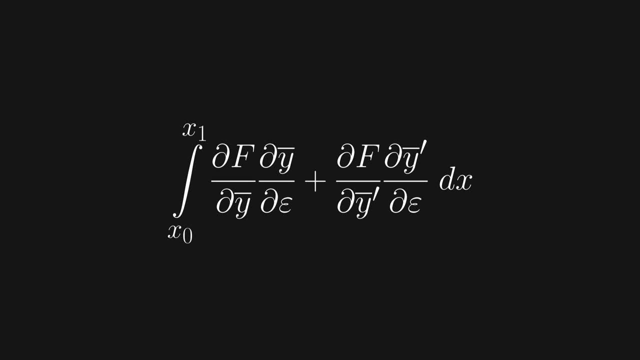 plus partial f, partial y-bar, prime times. partial y-bar prime. partial epsilon. Referring back to our definition of y-bar, we can simplify this again as: partial f, partial y-bar times eta. plus partial f, partial y-bar, prime times, eta prime. I now want to draw your attention to 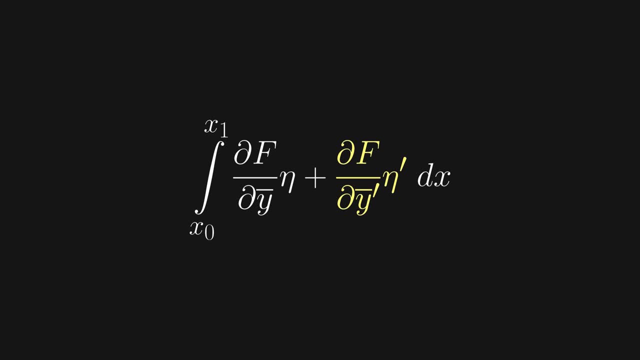 this term partial f, partial y-bar prime, times eta prime. We can use integration by parts to break up this integral even further. We let u equal partial f, partial y-bar prime and dv equal eta prime, dx. Then du equals d on dx of partial f, partial y-bar prime and v. 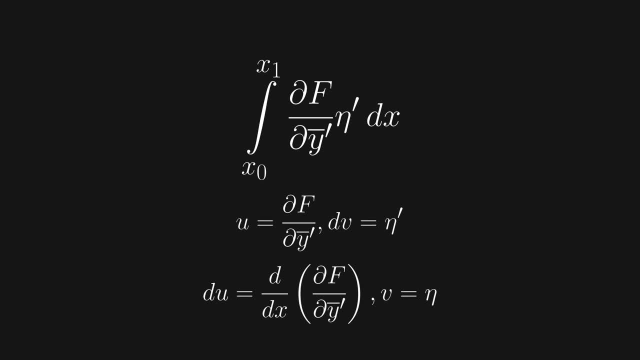 equals the integral of eta prime, which is just eta. By the rules of integration by parts. we can then rewrite this integral as: partial f, partial y-bar prime times eta from x0 to x1, minus the integral of eta times d. on dx of partial f, partial y-bar prime dx from x0 to x1.. 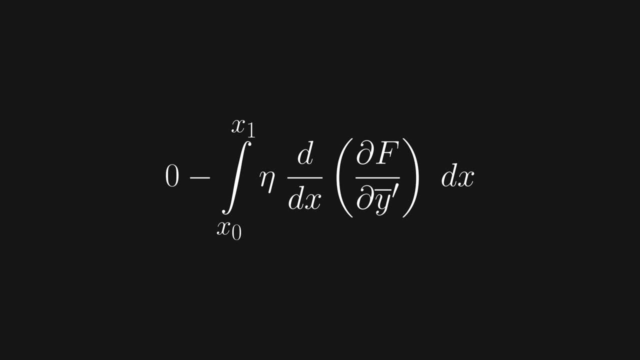 Notice that the first term becomes zero, since eta of x0 and eta of x1 both equal zero. If we plug this back into our original integral and factor out the eta in both terms, we get the integral of partial f- partial y-bar minus d on dx. partial f- partial y-bar prime times. 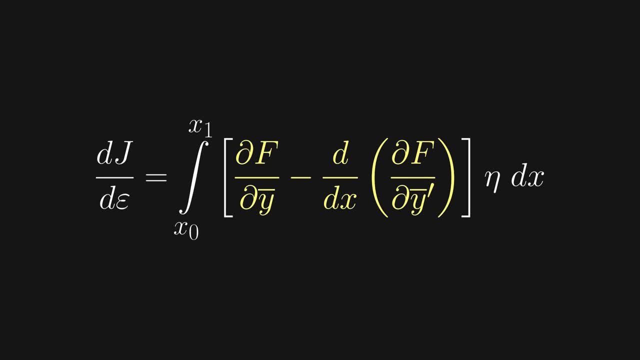 eta For our integral to be equal to zero. generally, we need this term to be equal to zero. This leaves us with the Euler-Lagrange equation. It is arguably one of the most important equations ever and it completely revolutionized mathematics and physics. As a summary, 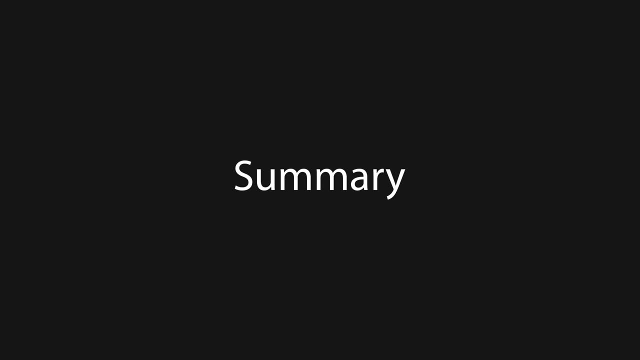 today we learned what it means to optimize a function, what a functional is and some of their applications, how to optimize a specific type of functional and hence derive the Euler-Lagrange equation. I don't think I'm quite ready to do a series on calculus variations. 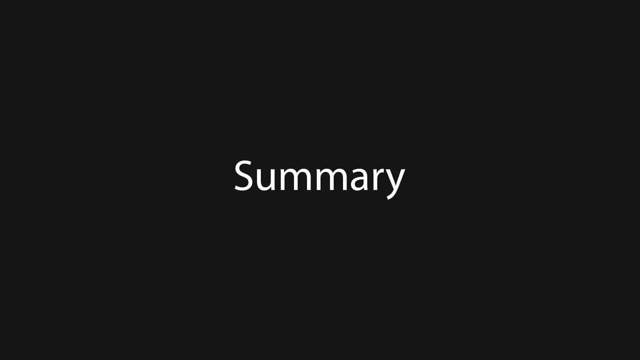 but I do plan to do a couple of worked examples with it, so let me know if that's something you'd be interested in. If you have any questions or spotted any mistakes, feel free to leave a comment. Thanks for watching.